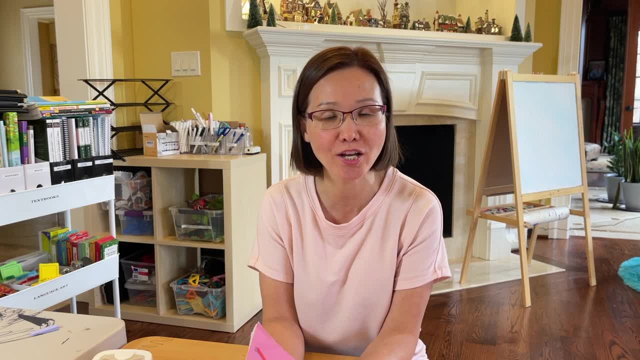 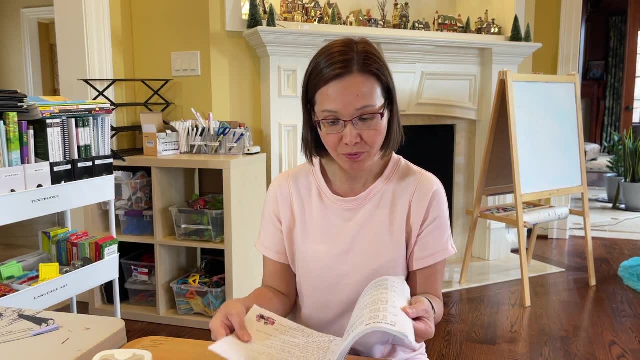 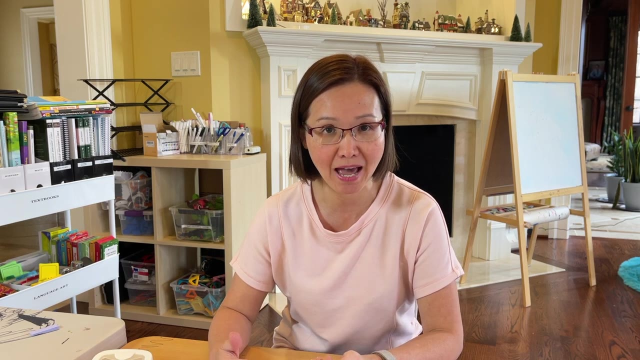 hi, welcome to my channel. today i will share with you how i do math lesson with my son and today, specific, we will learn about the money math. the reason why i want to talk about money math is because a couple weeks ago, when i start teaching him the math and i'm asking him to use the money, 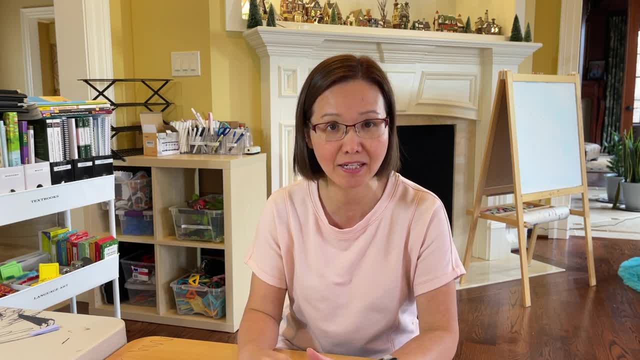 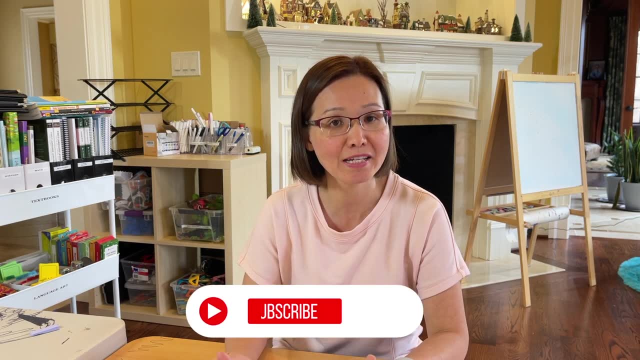 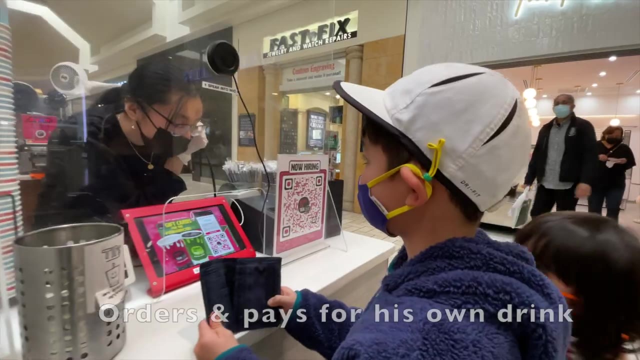 and he has a hard time doing that. he was able to do math on the paper beautifully perfectly, but when it's applied it to the money of the real money or the paper money, he could not do it at all and it's very intimidating for him and he's shy and he's he nervous. so i think maybe this: 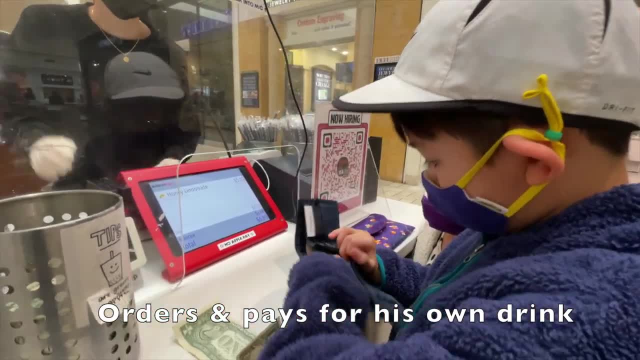 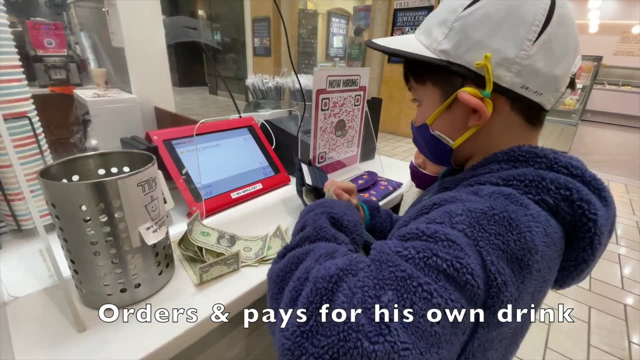 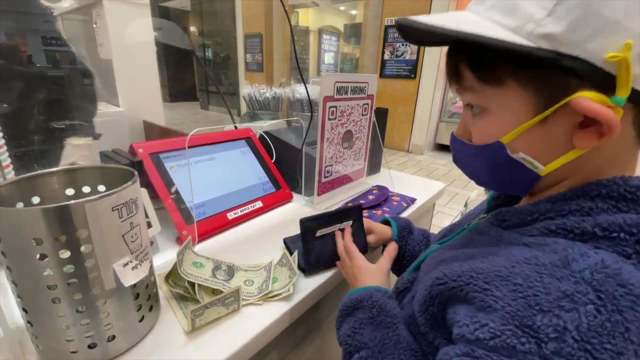 is a good opportunity for me to slow down and teaching him how to use money at the same time, how to apply his math to the real life, and i think it's important for me to taking time and give him opportunity to practice and seeing we are on the math lesson a couple weeks for like. 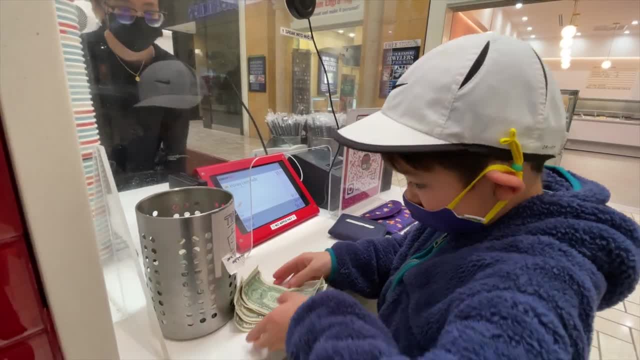 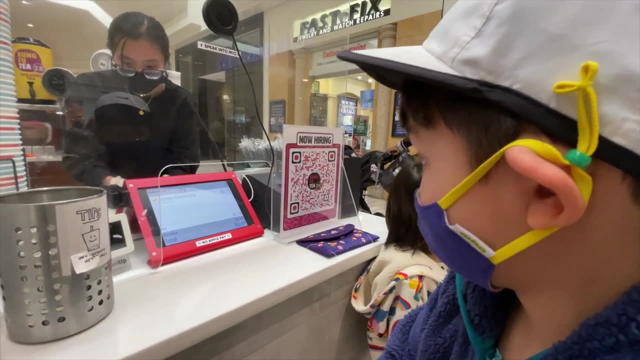 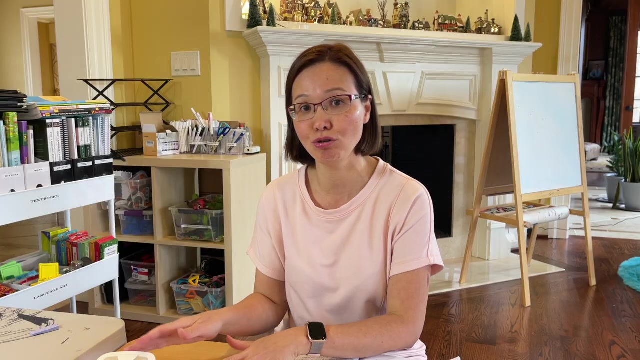 i think three weeks now and we just got it done, and this week is the last, last, final lessons, and i want to take this opportunity to share with you how i teach him math lessons on the paper, on the workbook and on the test book, and then apply it to the real money. so here i have. 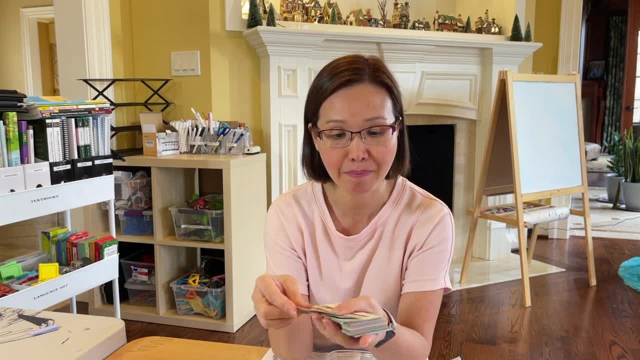 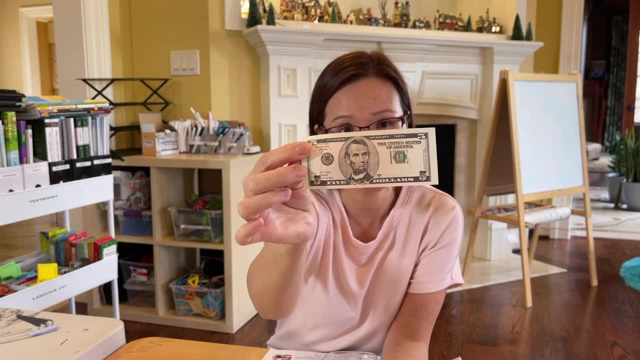 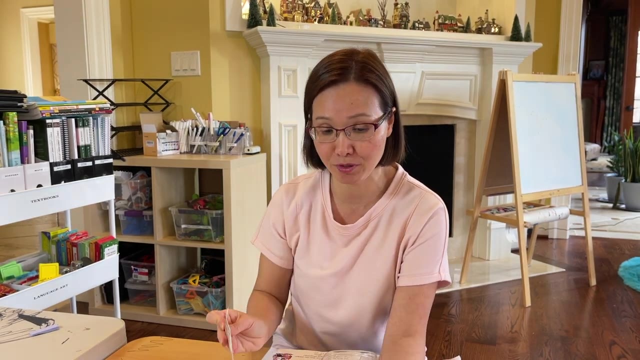 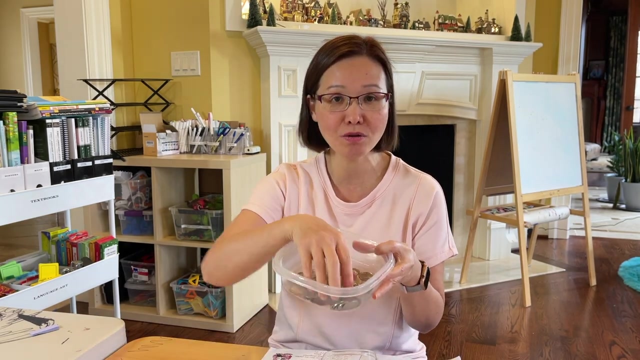 what i have here here is um, the money, the paper money. this paper money is really, it's thick, it looks real and close to the real money. so if there's no confusion for the kids to learn, um from this paper to the, to the real money, the fifty dollars right here, it's beautiful. also, i use the coin. i use a real coin. 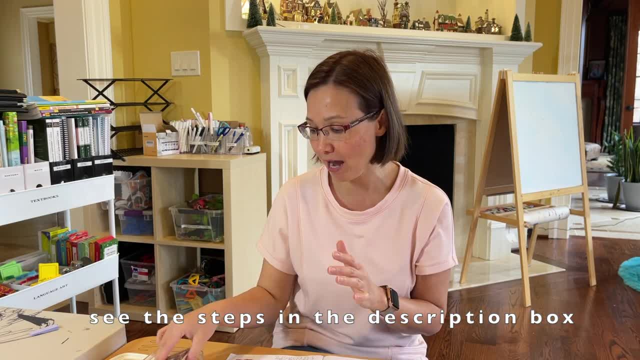 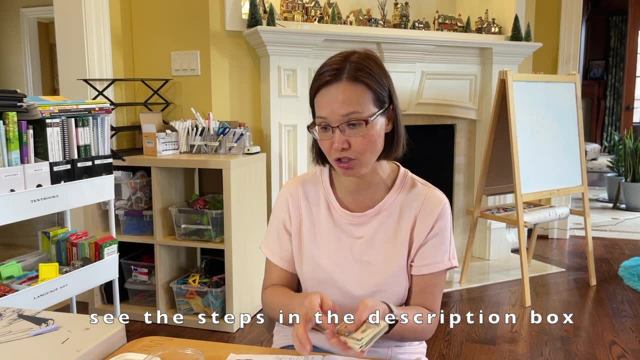 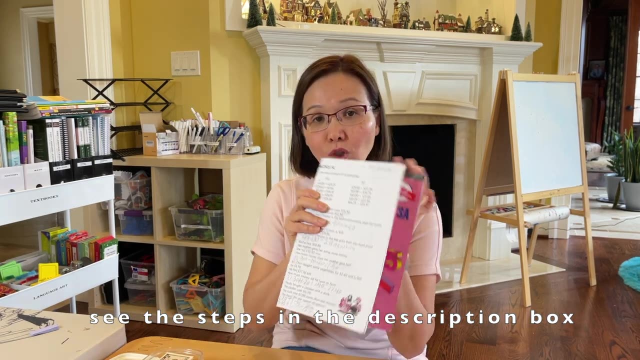 this is how i teach him. first of all i teach him how to short the paper and then i teach him how to short the money out. like five dollar go with five, one month, one dollar, but one dollar, ten dollars, will go with ten dollars. so i ask him to short it out on the table and then he will look. 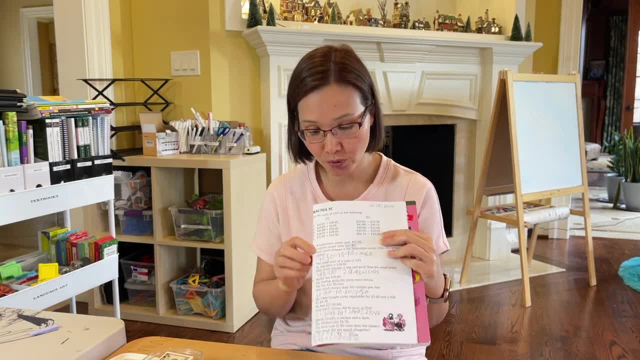 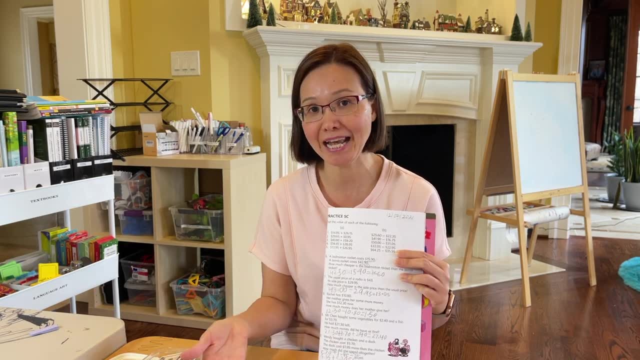 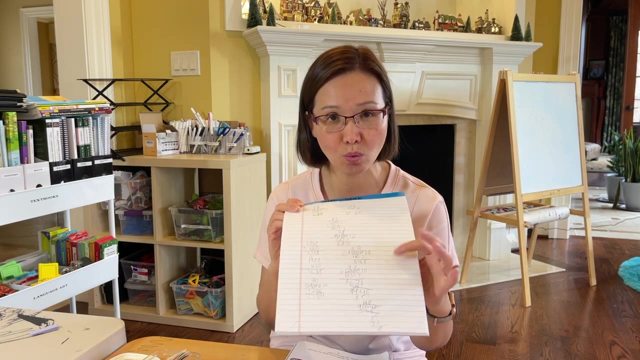 into his textbook or workbook. and what he's gonna do is he gonna convert this math problem into the money, pick out the money and do the and do the calculations. after he's done with his calculation with the paper money, what he does is he gonna go to his book or his, his paper right here. he gonna 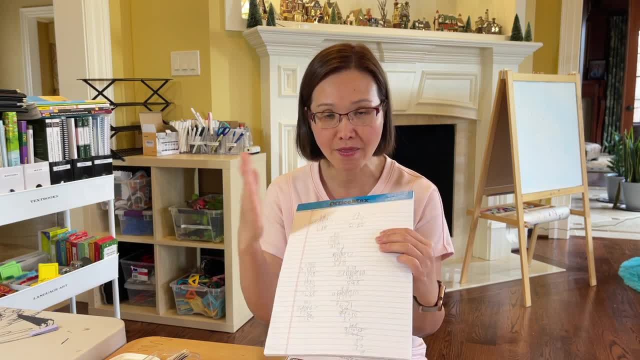 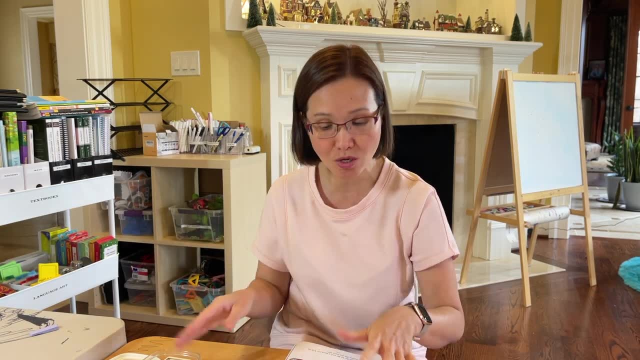 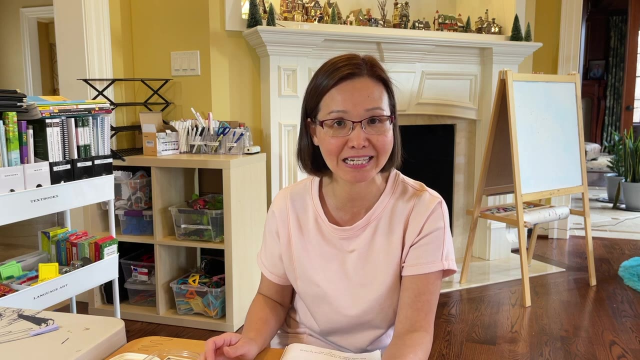 do the. he gonna test his math to make sure this math on the paper is matched with the paper money. after he done with that, he can write down his answer right here. if if he doesn't have the match number, the math result, he have to retest them. he either have to be done with the money. 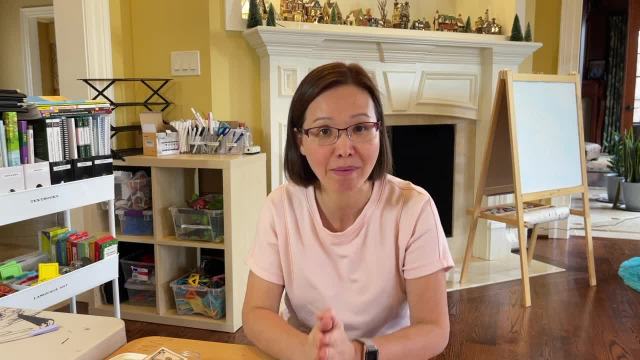 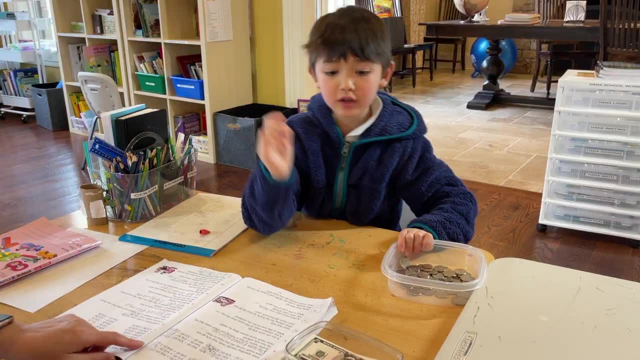 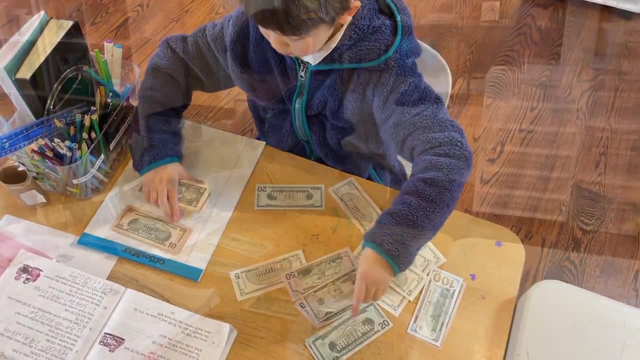 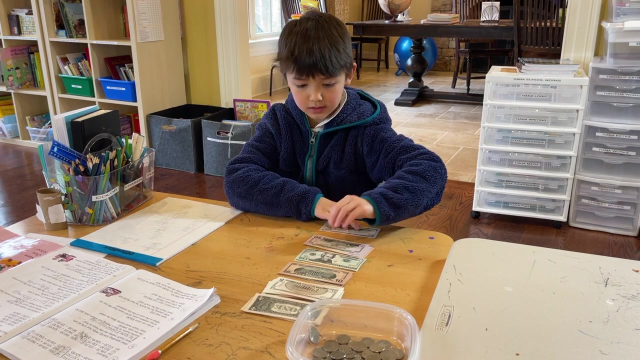 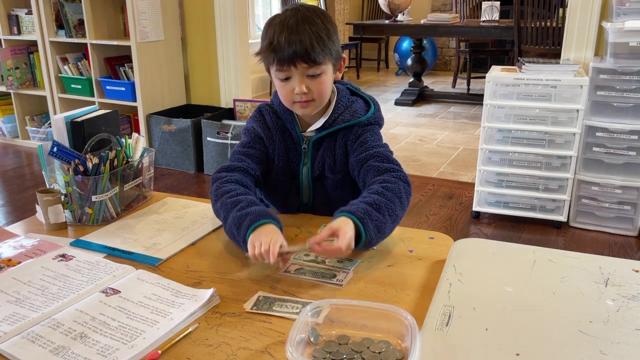 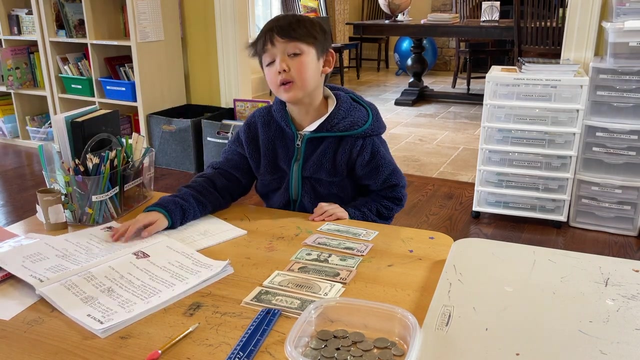 or with his math on the paper again. so i'm gonna call my son and we're gonna start to show you how do we do this. remember how to do this? so short it out, short it out, that goes next. and good job, my berries. so fourteen dollars. we don't have a four dollars, so we make a four dollar out of one dollars. 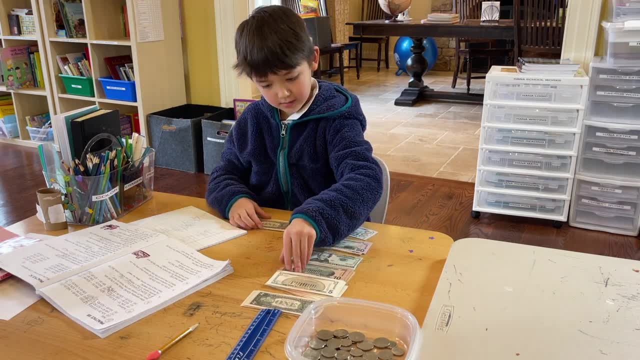 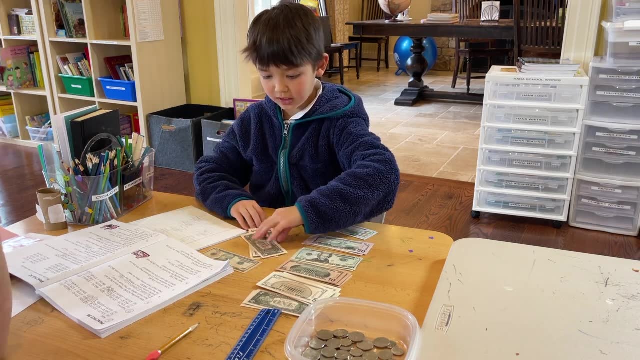 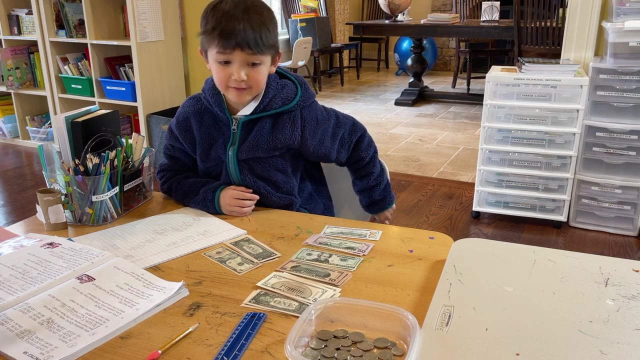 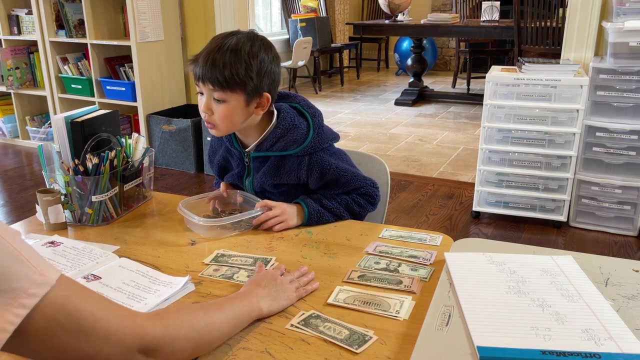 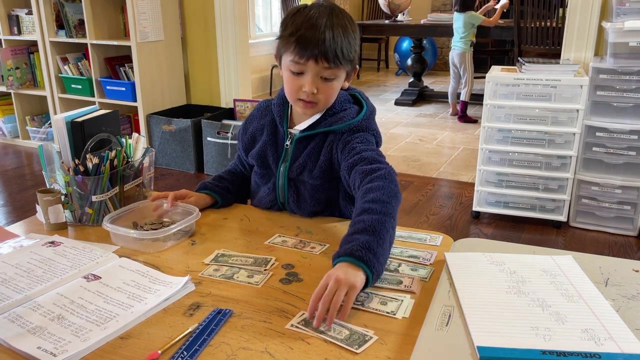 and to use this in less money, we use a ten, because you're not doing five plus five plus five or ten, so fourteen and eighty five, eighty five cents, eighty five plus two dollars, twenty six dollars. so we need a five dollar, one dollar, and we need a twenty dollar. 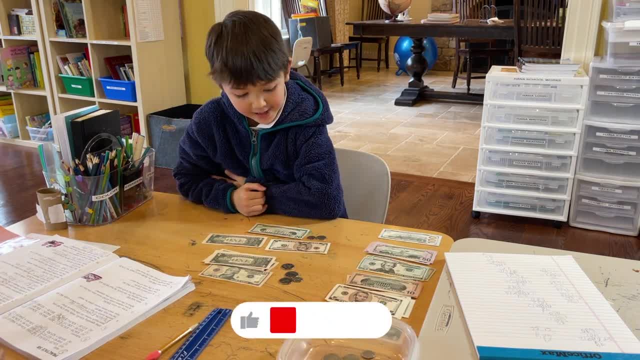 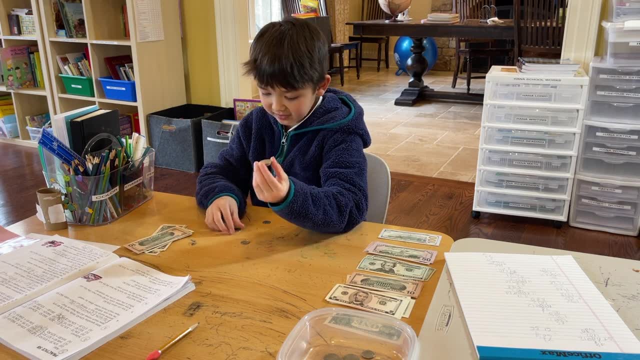 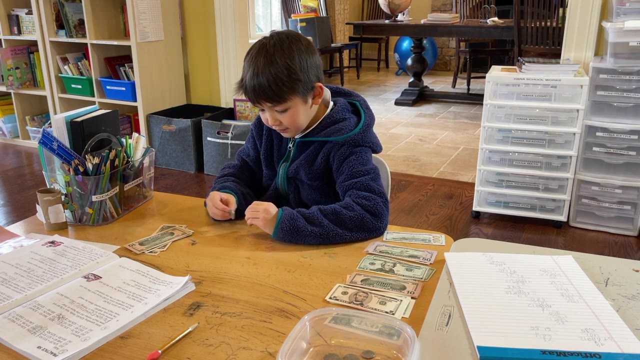 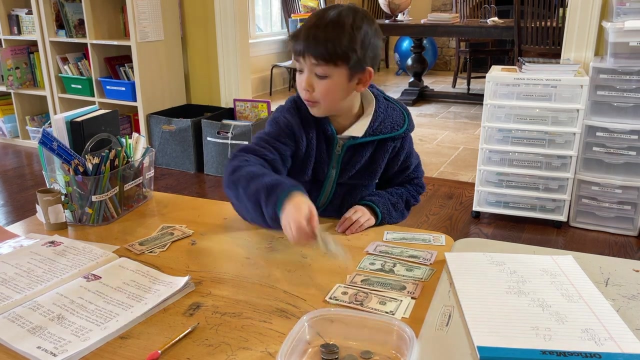 then we have fifteen. now we have to add thirty plus ten equals four, three quarters. seventy five cents plus ten equals eighty five cent plus five equals a hundred cents. that's one dollar. so i will put this away and one dollar we have. we have forty one dollars. 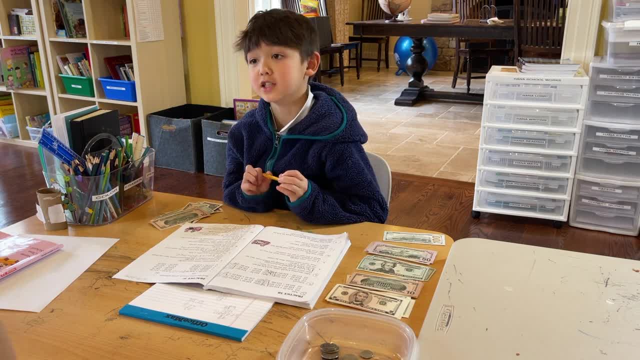 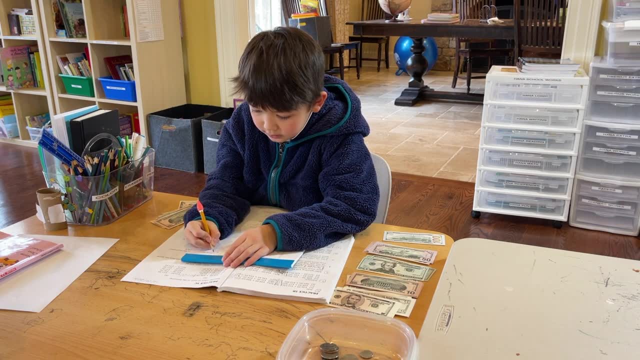 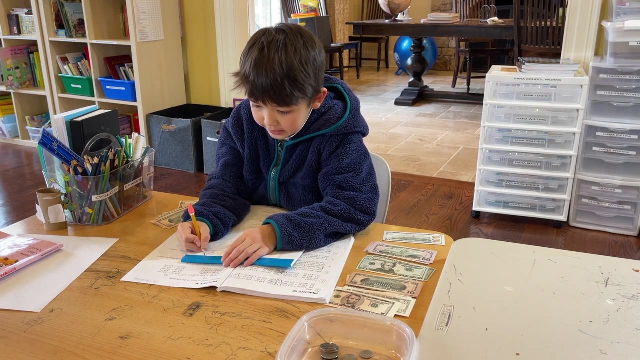 41. so, and we put this away one dollar and we have forty one dollars, we have 44. test to make sure this is correct: $85 plus $26.15.. Zero, $41.00.. Is that correct, $41.00. 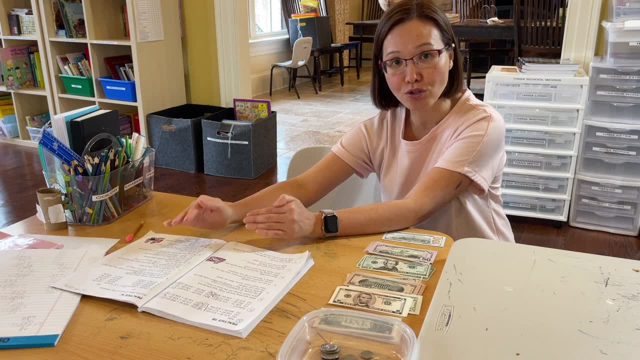 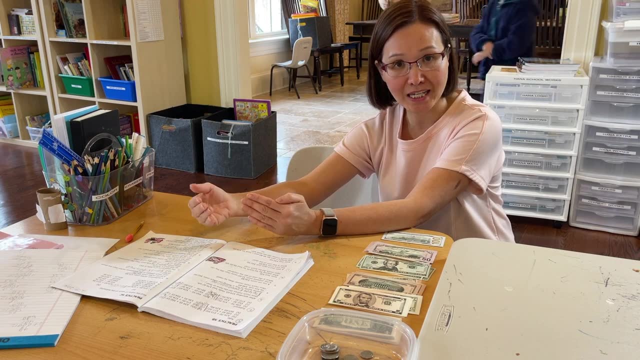 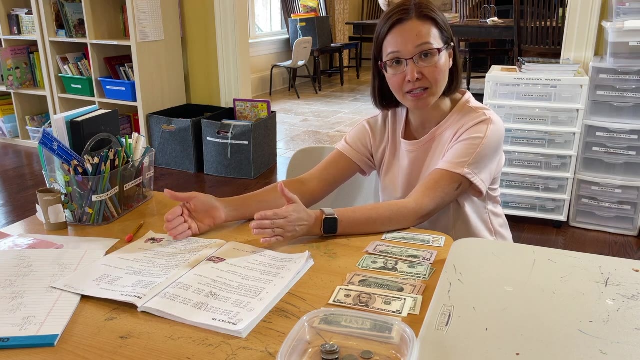 That's correct. What we're gonna do now is continue doing this lesson with the timer, Using timer to reinforce the focus and the discipline that he needs to stay in the timeline. That's how to improve his math skill at the same time. But if he cannot do it, 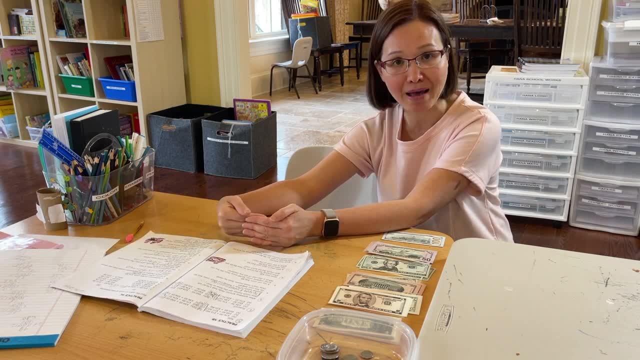 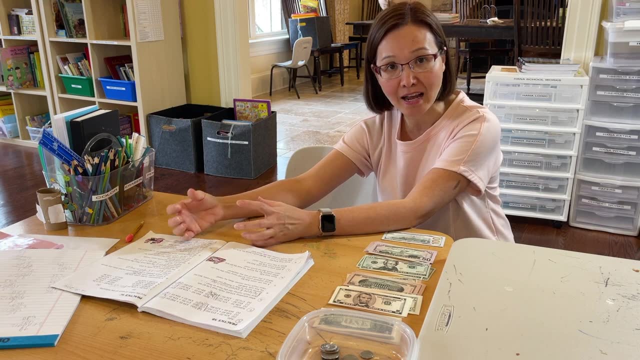 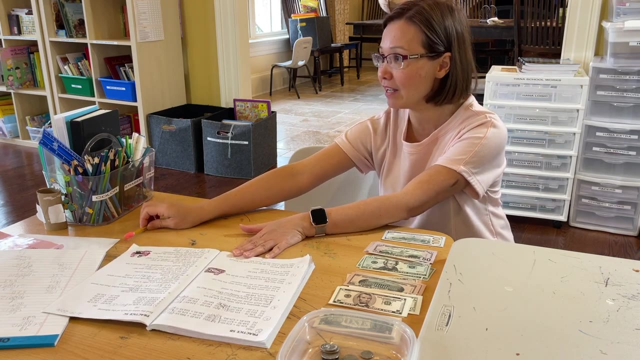 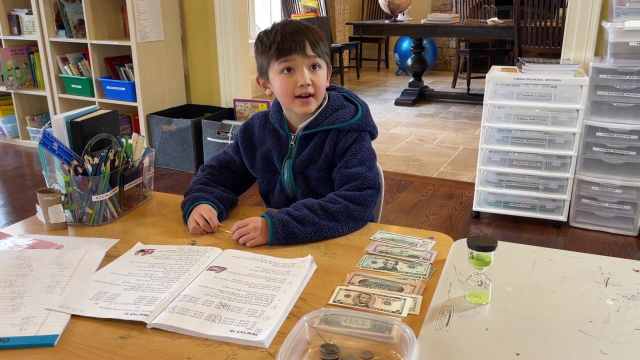 it's okay too. It just gives me the feedback that he needs to practice more, Or maybe he needs to break it down smaller steps to practice more. I'm gonna put the timer on right now and see how he does. Okay, let's come back here. $29.65 plus $0.95.. We have 20.. We need a 9.. So we have. 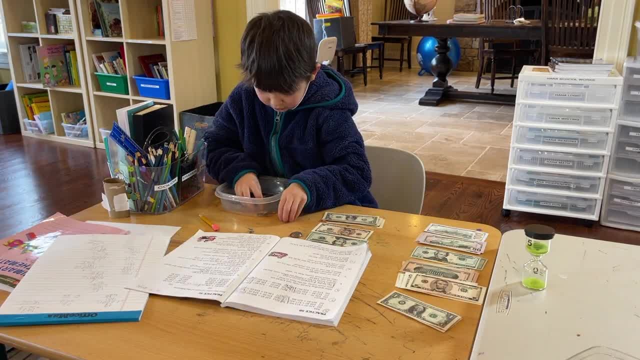 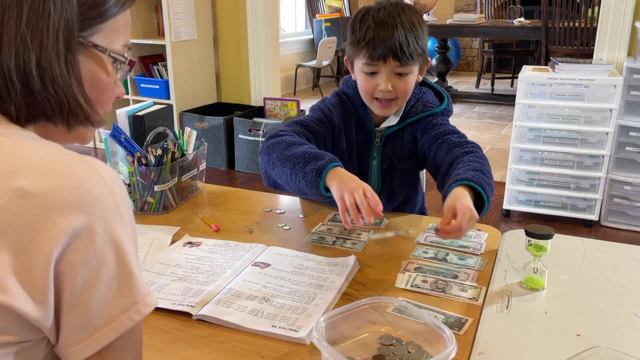 5.. 5 and a 10. Then we need 95.. So we're $1.00.. Bye, bye, Look, look, look, No, because that was $1.00.. No, that is $0.05.. Okay, keep going ahead. 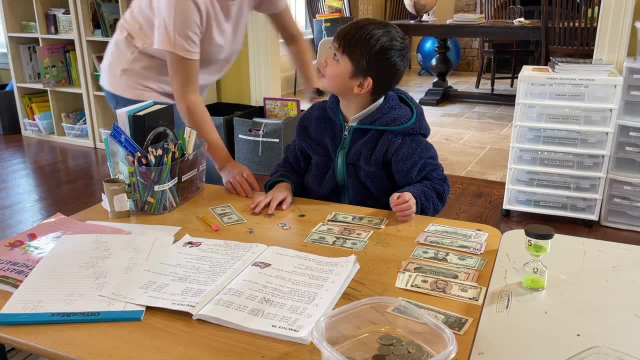 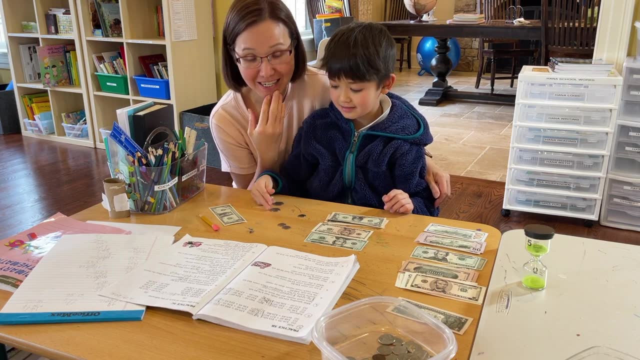 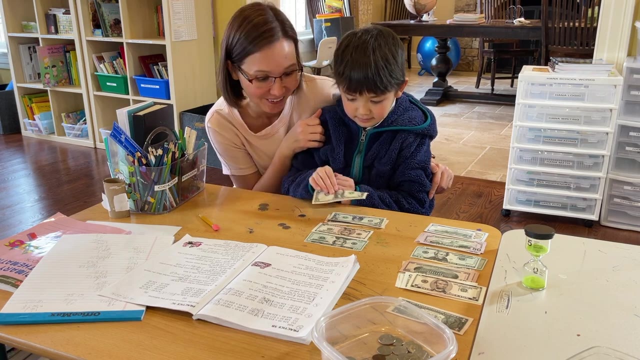 Because I've got. I've got six quarters. So I just, I just could not stop myself that I had to stop him. But I can recognize that I let him be because this is a good example that he had to redone his math later on. So I should stop. 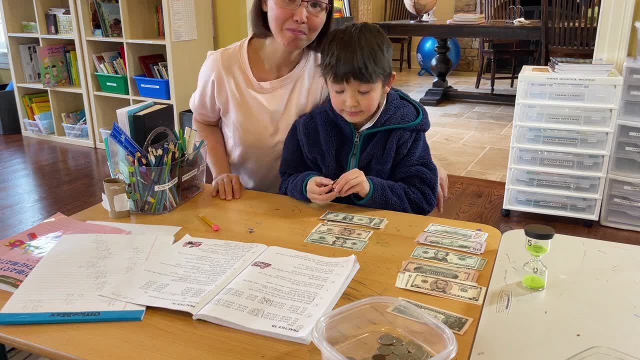 myself that you know this is a one of the owls. you know, as a mom mistake right, That we just want to come in and fix something. So I'm gonna stop myself. I'm gonna stop myself, I'm gonna stop. 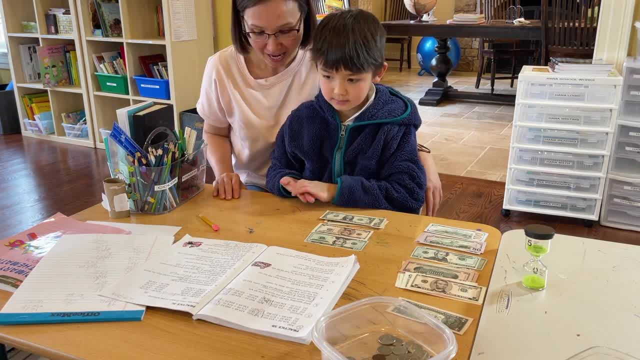 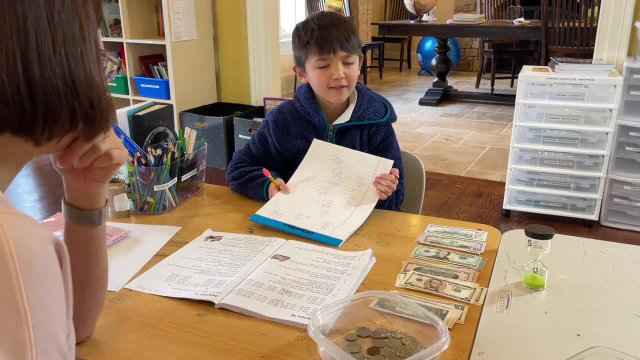 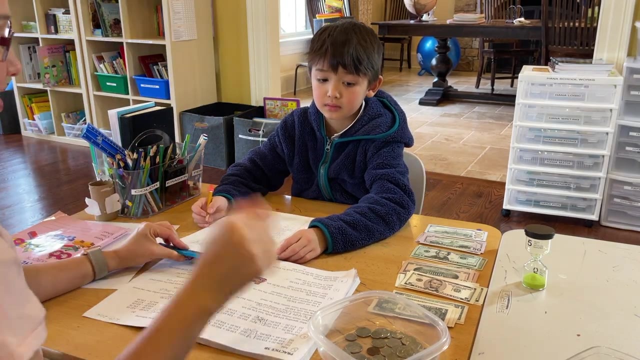 the problem. So I was jumping over him. Let's see if he can figure that out and do this math correctly. So there was Okay. First we have to do problem two: test them. I nearly forgot, I'm sorry, I didn't cross off my hands. All right, so now I'm gonna test you. We're gonna redone your. 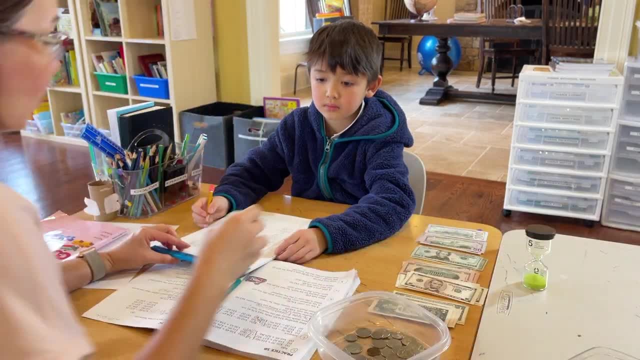 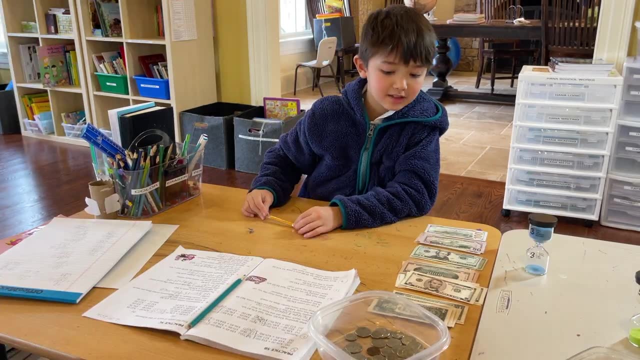 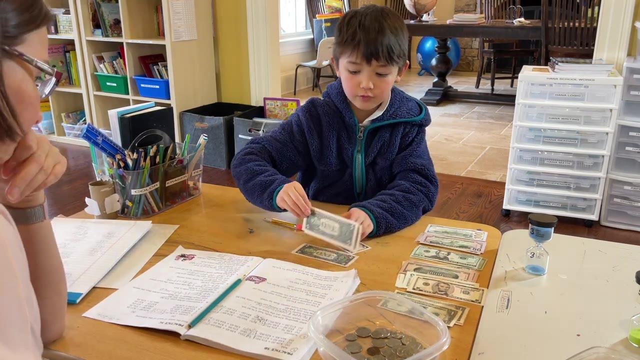 math in three minutes. Okay, let's do this. Are you able to focus now? Uh-huh Ready- $29.. Okay, $29.. Keep testing your problem. Okay. so I think that's it for today for us. Thank you for joining us. 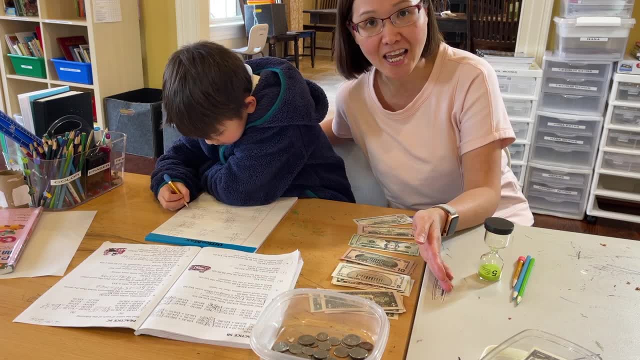 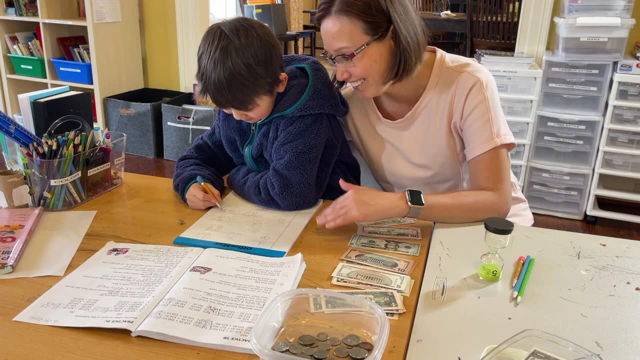 with the math lesson today. I hope you have a wonderful day to whatever you're doing and I will see you next time. And we forgot to video the rest. Yes, we did. We forgot to click on the recording button for the second. 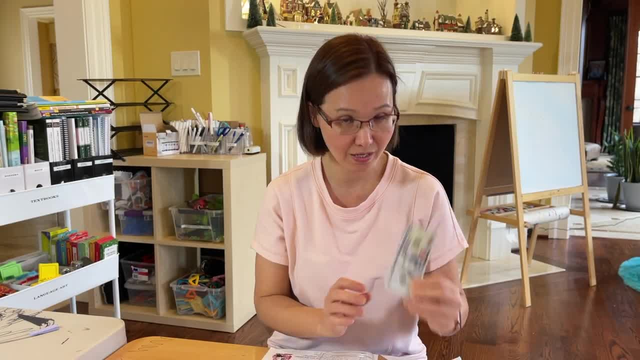 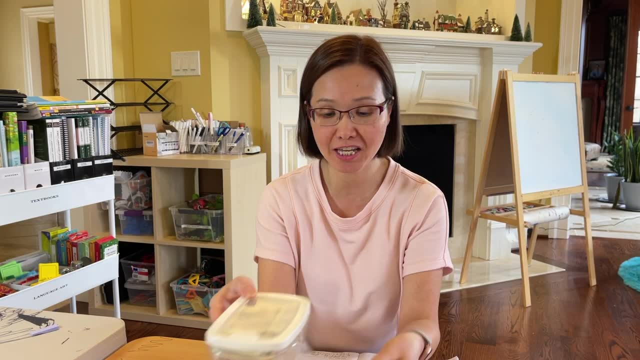 Subtraction lessons. So what I bought, I bought from the. I bought the paper money. The paper money is from um Do it. I could keep the two box together like this. This you know, like you don't have. 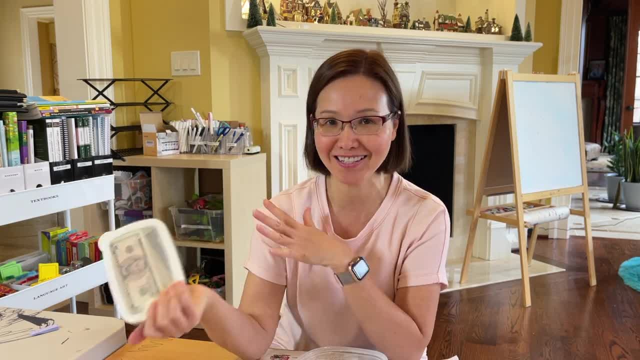 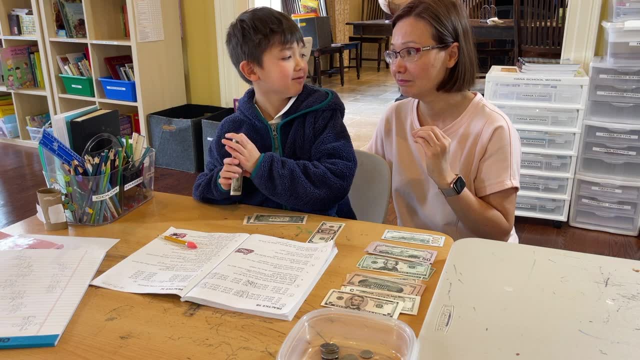 If you see me, uh, you won't see fancy boxes, other stuff, And discipline is the answer to everything. And don't forget, looking at an ancient fossil is the answer to everything, Especially cake, Uh, Hooray, More words. 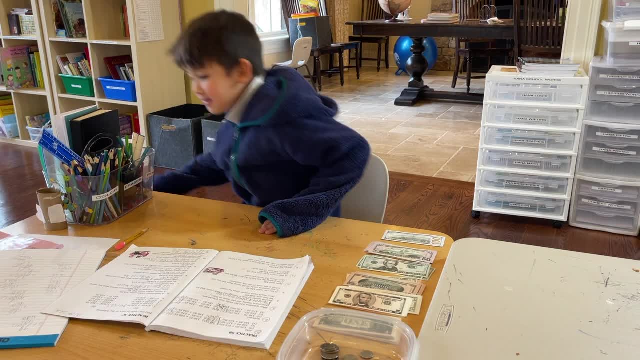 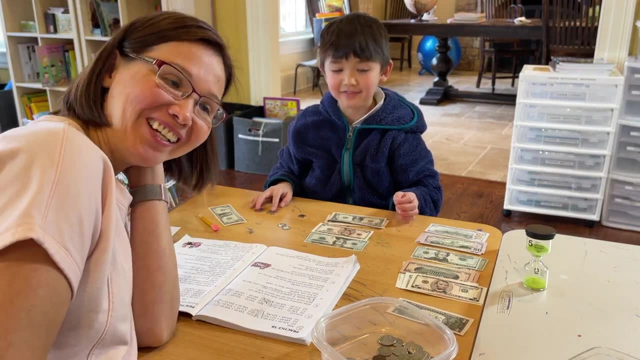 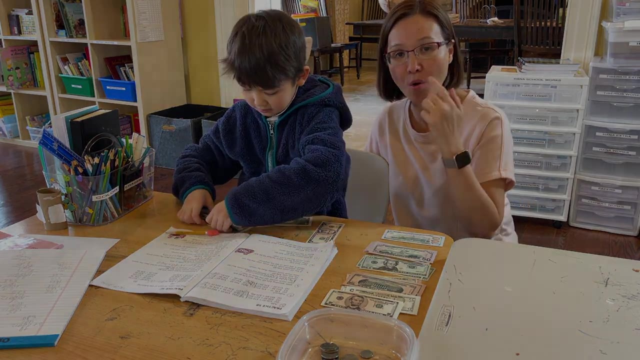 I love math, That's my favorite subject of the day, And it never includes drinking water for three hours. So Because I've, I've, got, I've got, I've, I've, I've, I've, Give him the timer to speed up, and when he does that, it requires more focus. 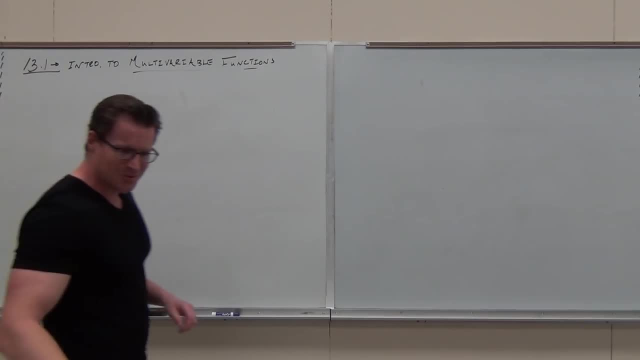 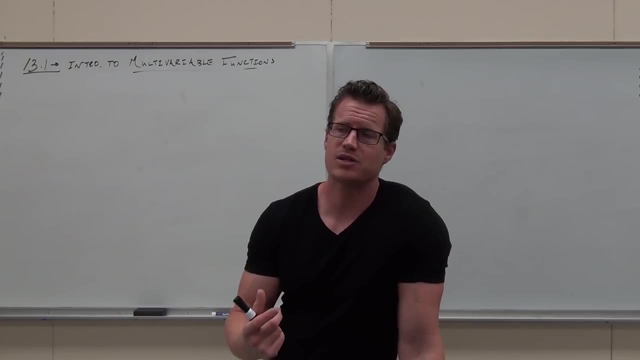 So, new section, new chapter, some cool stuff We get to talk about, finally, some multivariable functions, how these things work, how they look and especially how the calculus relates to them, Because when you start dealing with more than one variable, what I mean by that is more than one independent variable. 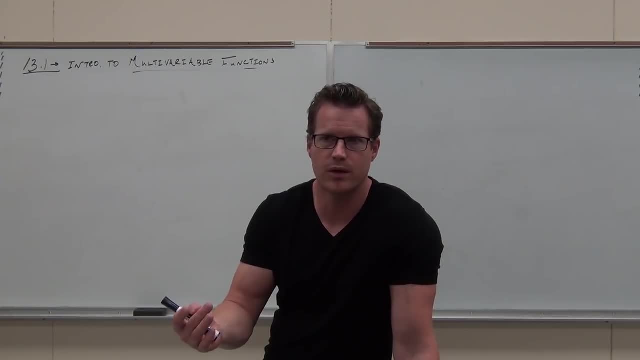 things get kind of screwy, like what's a derivative when you've got more than one independent variable. That's what we're trying to answer, and we start that with just an introduction about what these things do, what the domain is and how they work. 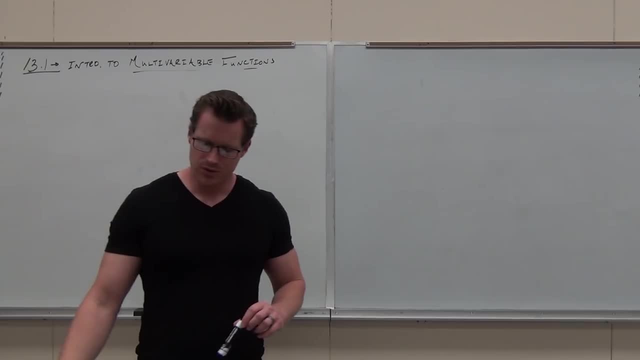 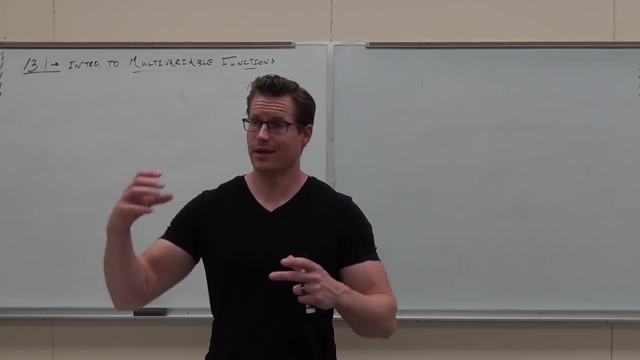 So we're used to talking about functions, but we're used to talking about functions in just one variable. Now please get this straight: When I say one variable, I mean one independent variable. so, like with X, The dependent variable Y, there's always only one dependent variable. all right, 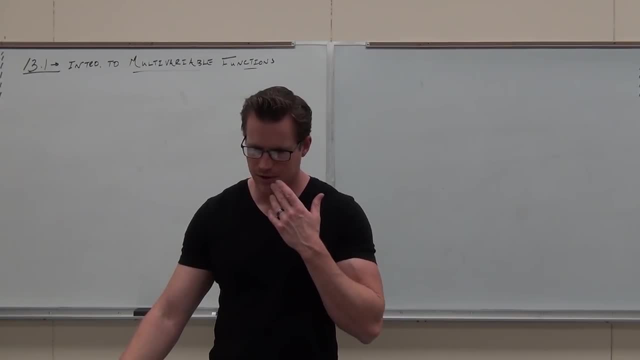 But now we're going to start saying, okay, what happens when we have more than one independent variable? Well, there's good news and bad news. The good news is that the same stuff basically works. You still have a domain, You still have a range.